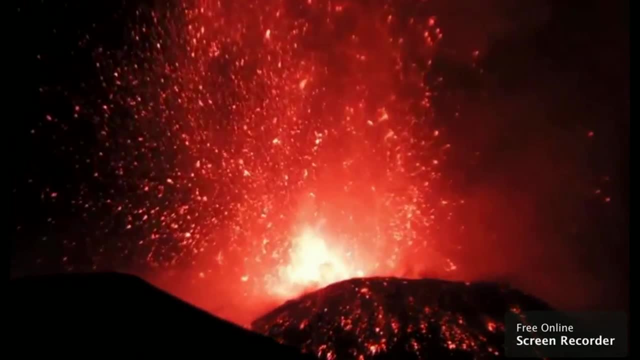 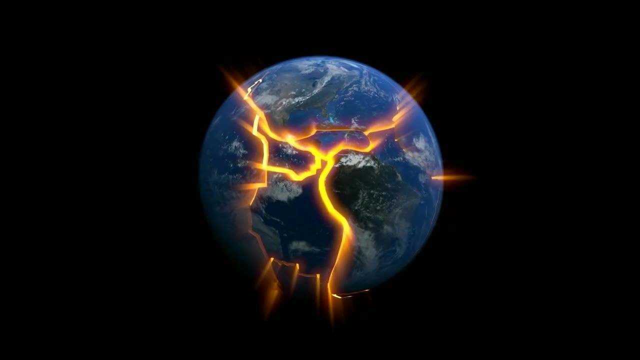 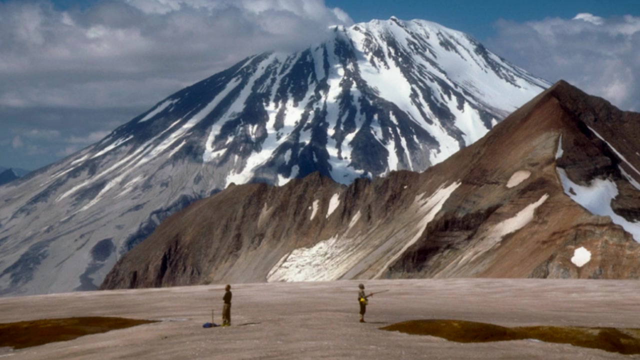 erupt onto the Earth's surface. Many volcanic mountains occur at convergent boundaries. Most of the Earth's active volcanoes are concentrated around the edge of the Pacific Ocean. This area is known as the Ring of Fire. Mount Griggs in Alaska is an example. It is 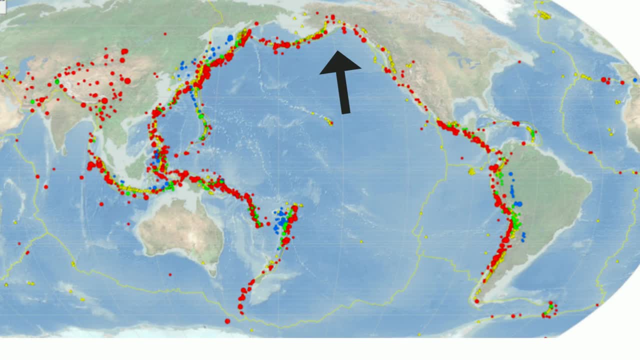 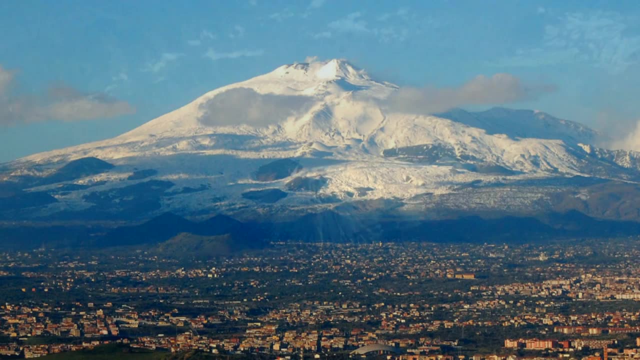 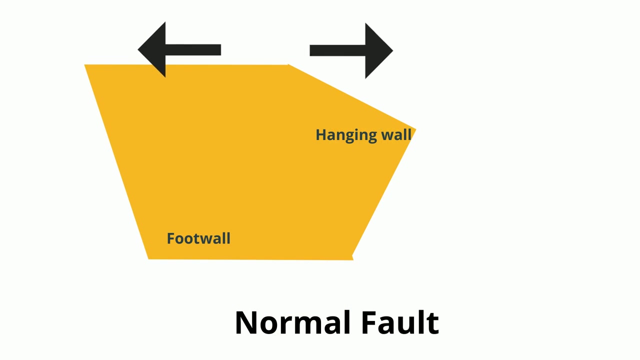 located on the northern rim of the Pacific plate. Other examples include Mount Fuji and Mount Etna. Fault block mountains form when tension causes the lithosphere to break into normal faults. At normal faults, the lithosphere drops down. The pieces left standing form a fault block. 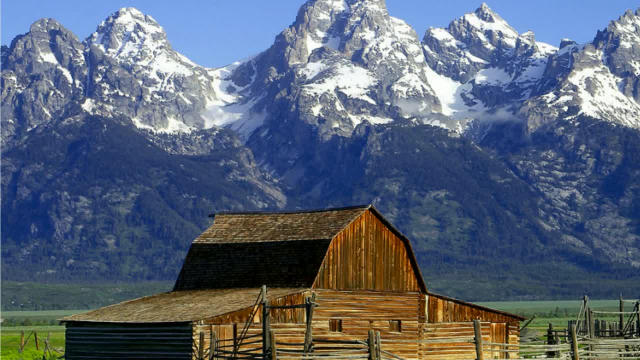 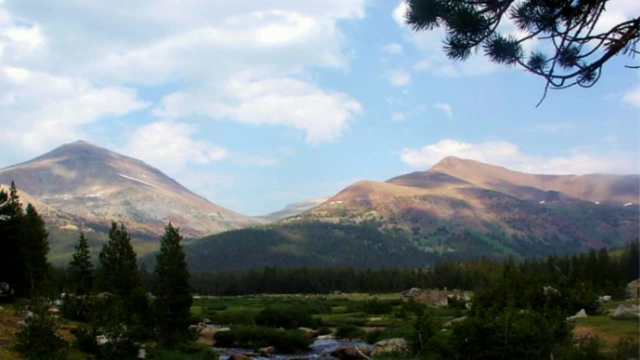 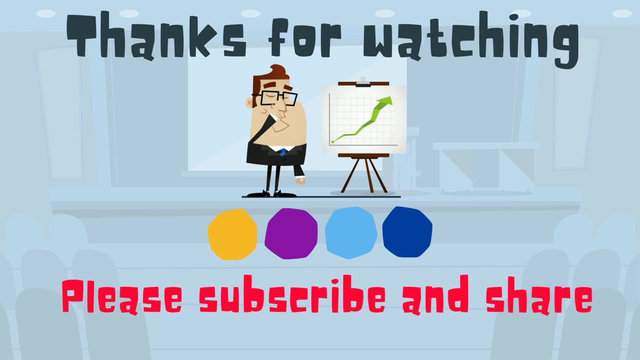 mountain- The Teton Mountains is an example- And the Sierra Nevadas. So I hope that helps with understanding different types of mountains. Thanks for watching. I'll see you next time. And MooMooMath uploads a new math and science video every day. Please subscribe and share. 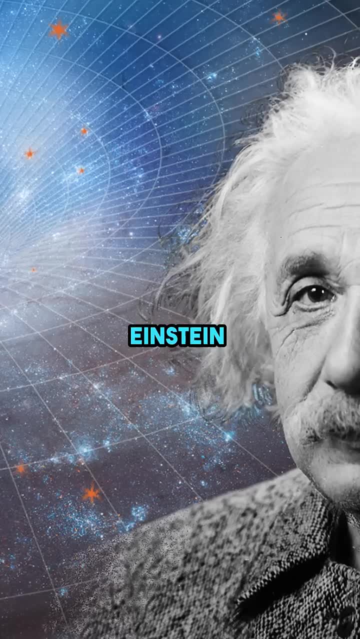 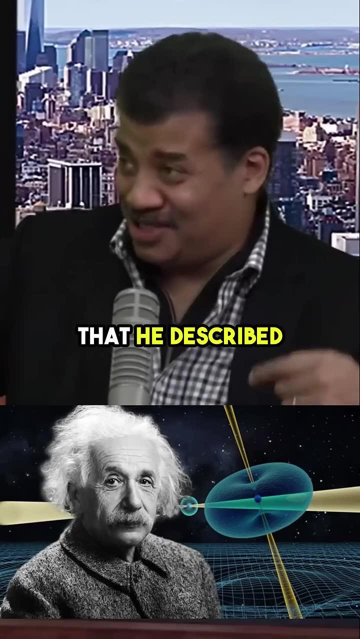 Einstein's gravitational waves. How was it finally discovered? Einstein, 100 years ago, gave a recipe for prediction of how you might be able to detect the kind of gravity that he described in his famous 1916 paper. To him, gravity was not a force. Gravity is the distortion in the. 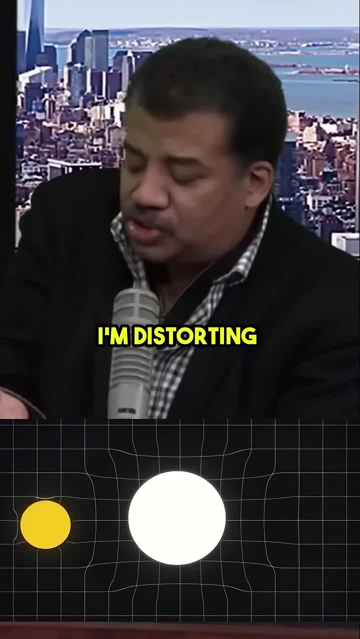 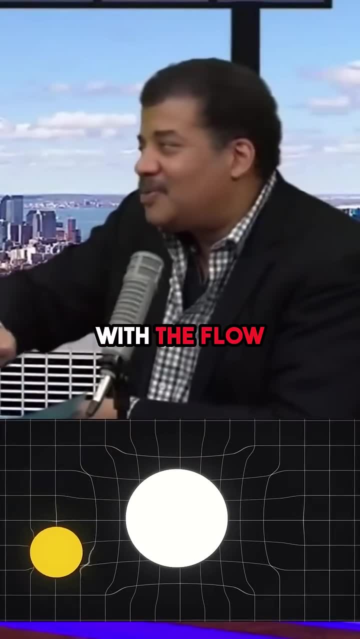 fabric of space and time. And if I have a massive object I'm distorting it deeply And some other object comes in the vicinity, it kind of falls into that distortion. So you're really just staying with the flow. And I think it was one of Einstein's disciples who came up with the phrase. 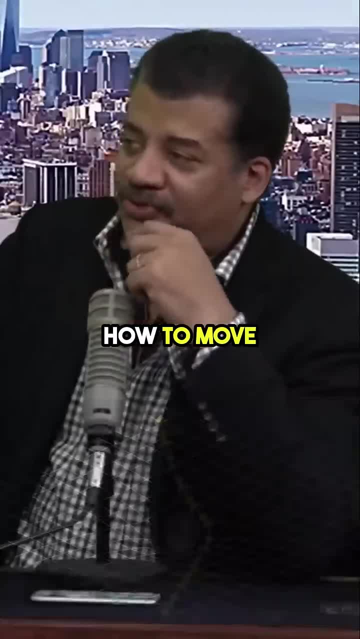 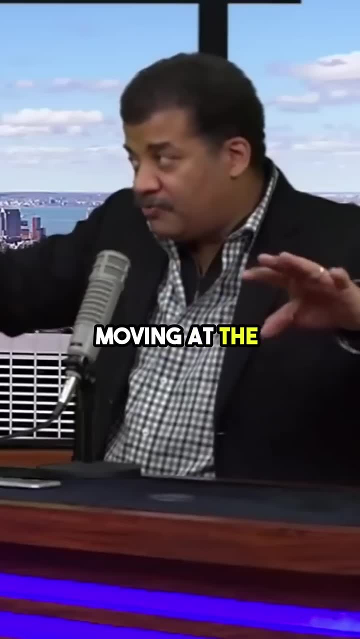 matter tells space how to curve, space tells matter how to move, And so now, if you have a disturbance in this fabric of space and time, it will emanate forth as a ripple moving at the speed of light. And that ripple that was discovered and announced today has been traveling through the 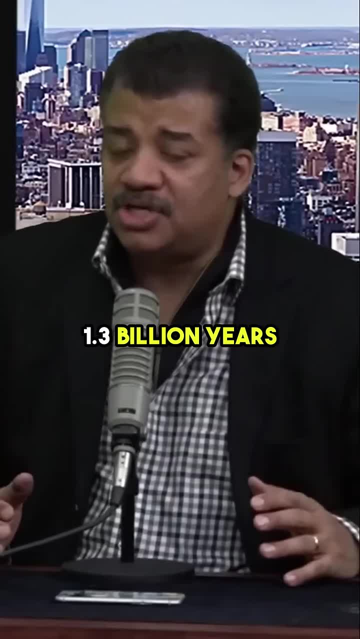 fabric of space and time for 1.3 billion years, And it is the record of the collapse of a double-edged sword. And it is the record of the collapse of a double-edged sword. And it is the record of the collapse of a double-edged sword And it is the record of the collapse of a double-edged.